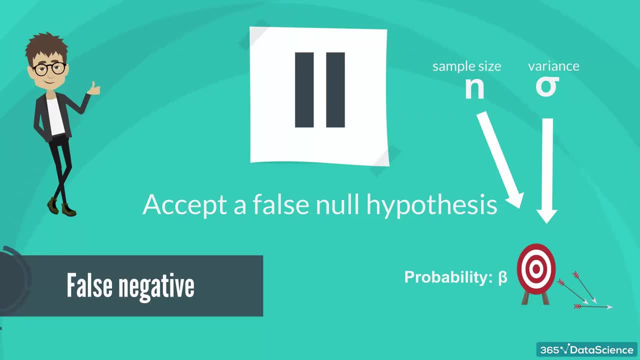 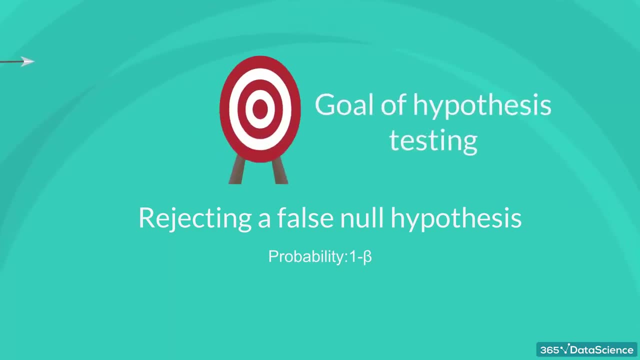 is considered a smaller problem. We should also mention that the probability of rejecting a false null hypothesis is equal to 1 minus beta. This is the researcher's goal: to reject a false null hypothesis. Therefore, 1 minus beta is called the power of the test. 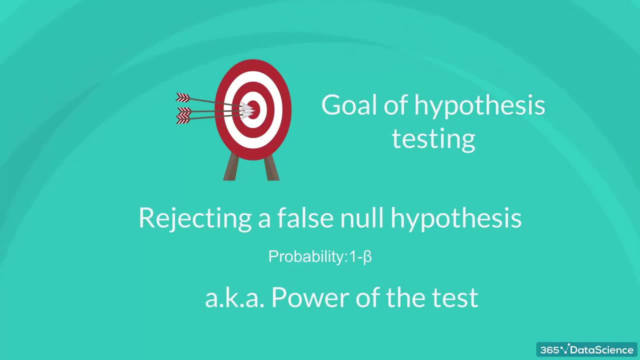 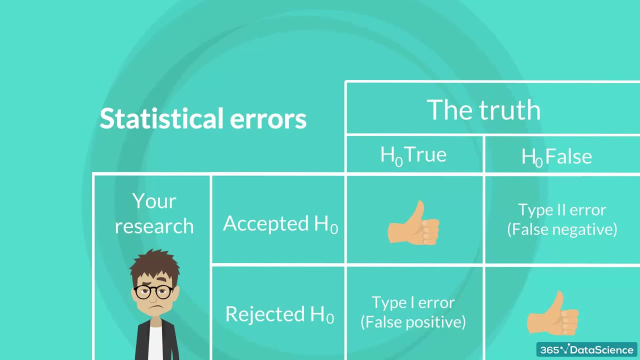 Generally, researchers increase the power of a test by increasing the sample size. This is a common table statisticians use to summarize the types of errors. Now let's see an example that I heard from my professor back when I was studying statistics in university. 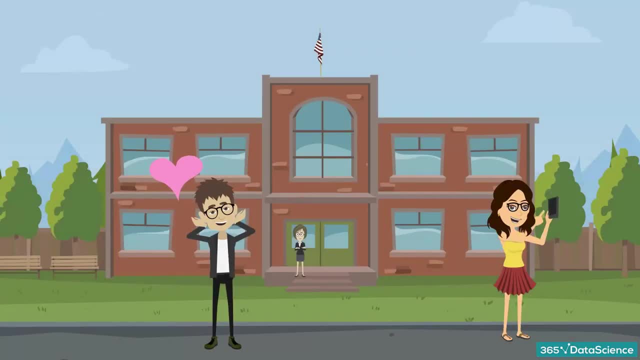 You are in love with this girl from the other class but are unsure if she likes you. There are two errors you can make. First, if she likes you back and you don't invite her out, you are making the type 1 error. 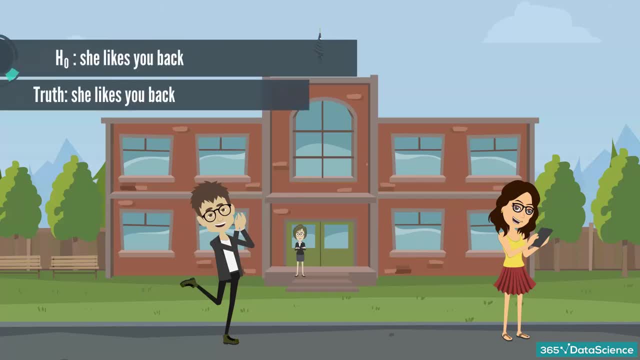 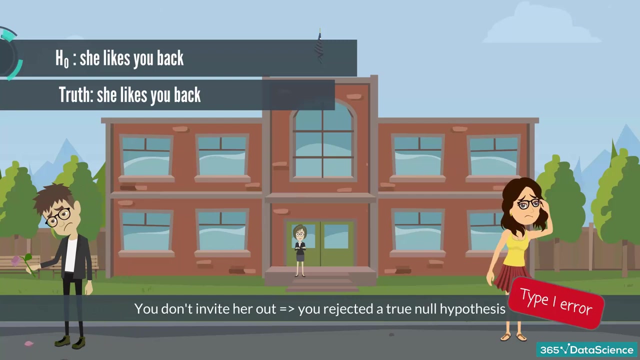 The null hypothesis in this situation is: she likes you back. It turns out that she really did like you back. Unfortunately, you did not invite her out because, after testing the situation, you wrongly thought the null hypothesis was false. In other words, you rejected a true null hypothesis and lost your chance. 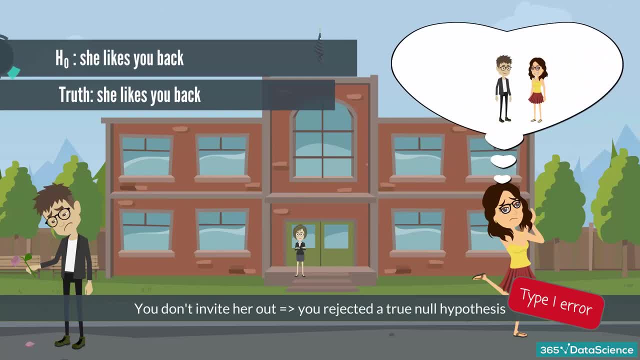 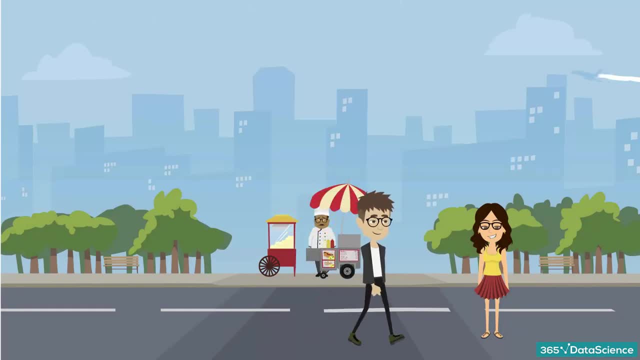 It is a very serious problem, because you could have been made for each other, but you didn't even try. Now imagine another situation. She doesn't like you back. She likes you back, but you go and invite her out. The null hypothesis is still. she likes you back, but this time it is false. 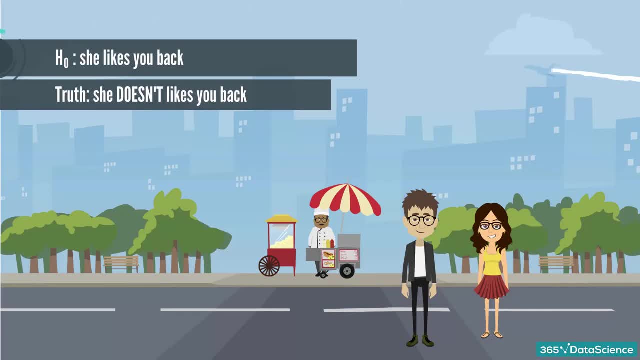 In reality, she doesn't really like you back that is. However, after testing, you accept the null hypothesis and wrongly go and invite her out. She tells you that she has a boyfriend that is much older, smarter and better at statistics than you and turns her back. 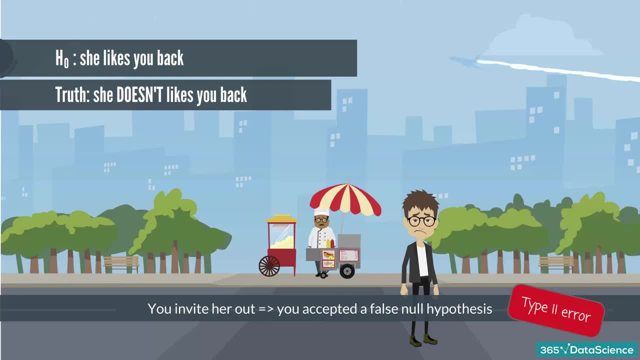 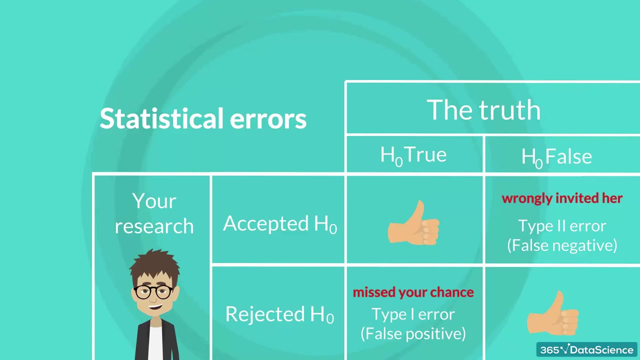 You made a type 2 error, Accepted a false null hypothesis. However, it is no big deal, as you go back to your normal life without her and soon forget about this awkward situation. Hypothesis testing is usually like that: You don't really want to make any of the two errors, but it happens sometimes. 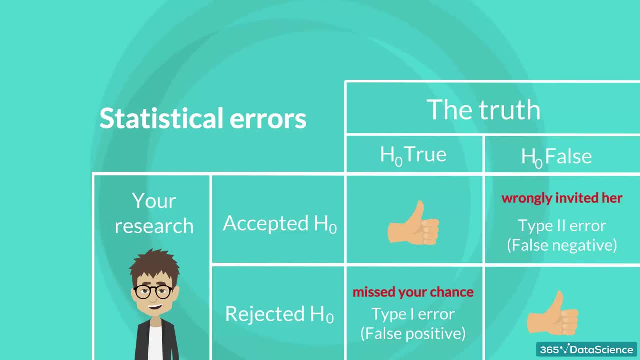 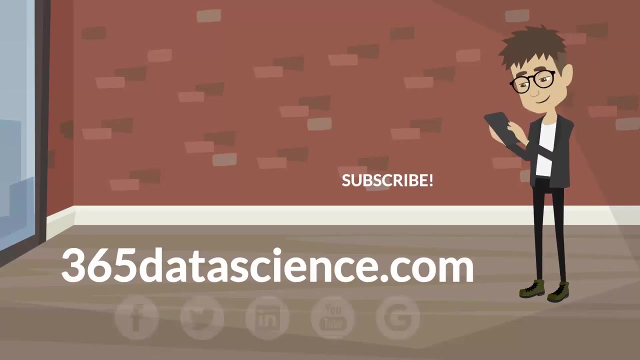 You should be aware that statistics is very useful, but not perfect. Alright, that's all from our love. slash life. slash statistics lesson. Thanks for watching. We'll see you next time.